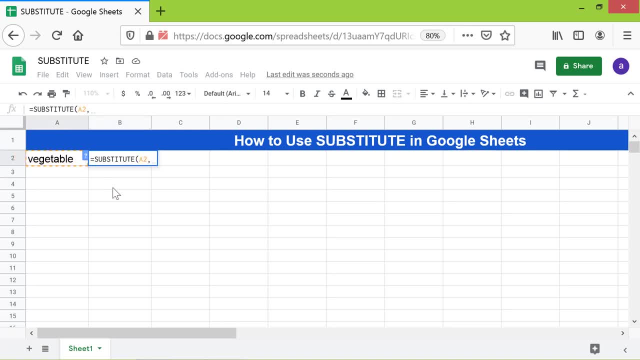 Type comma For SearchFor type E between double quotes. Type comma For ReplaceWith type E S between double quotes. Type comma For OccurrenceNumber type 3, because we want to replace the third instance of E with E S. 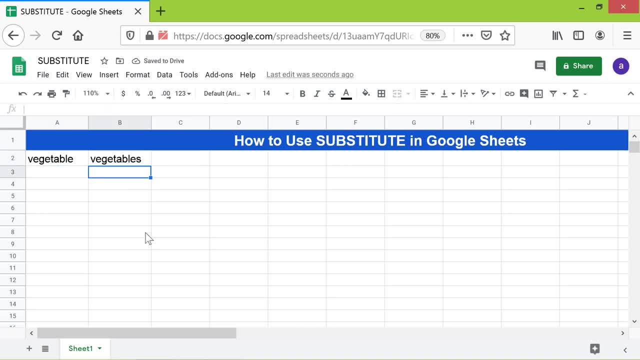 Press Enter. There you go. The Substitute function has substituted E with E S. Let's look at another example. In this we want all occurrences of the string to be replaced. Let me type the text in this cell: Type comma, Type comma. 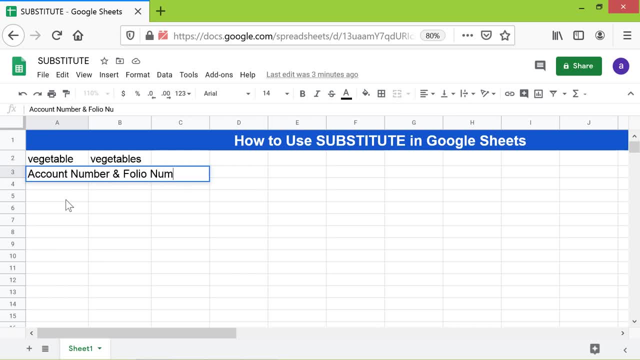 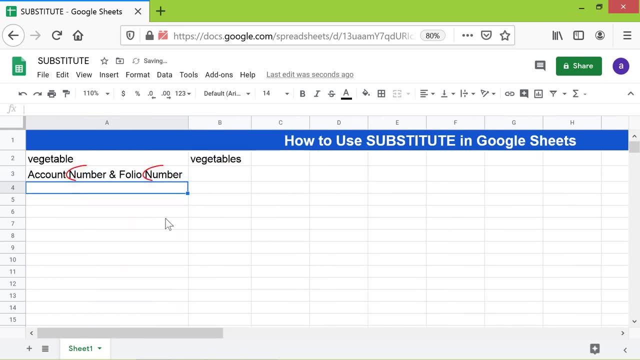 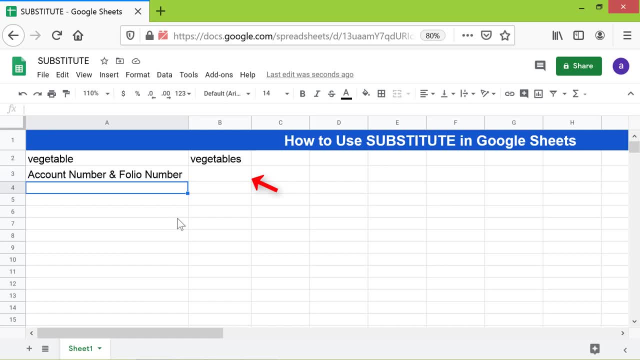 To be replaced by its abbreviation. Ok, the formula has returned the desired output. Moving forward, remember that Substitute is case sensitive. So what happens if I type the letter n in small case in the formula? Let's find out. 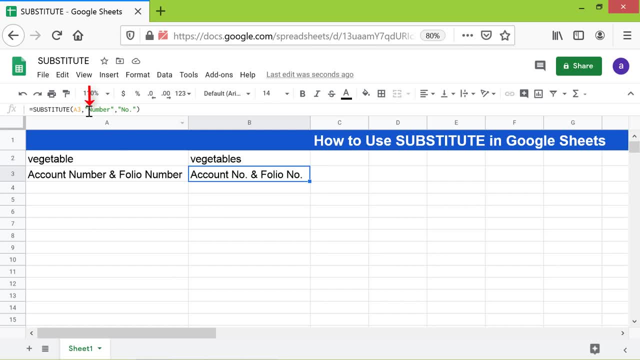 Replace the capital N with a small n. The Substitute formula has returned the original string Instead of the modified string, Because it could not find the text number with a small n. Alright, let me click this cell and change the formula the way it was before. 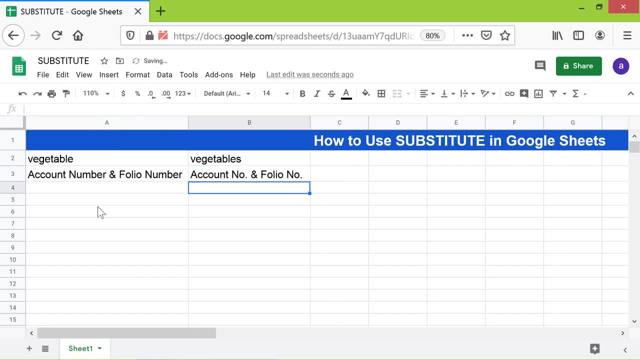 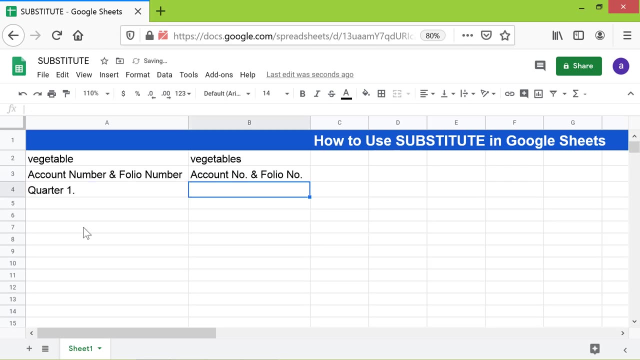 Ok, the output is correct and is the same as the one prior to changing the case. Here is another last example. Say you want to replace the period with nothing. To get this output for the replace with attribute.